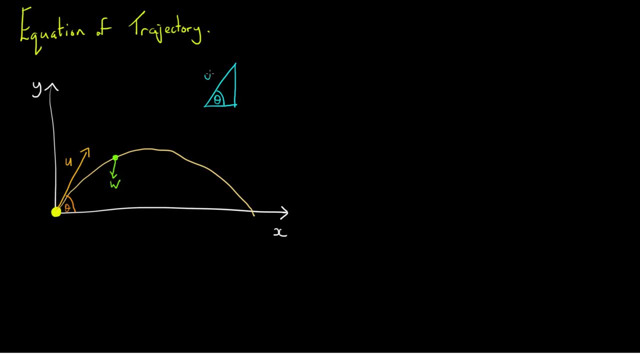 we have a triangle, that's angle. theta here, hypotenuse is u, and we want to resolve this to gain our initial vertical velocity, which is this distance, and our initial horizontal velocity, which is this distance. We give these u of y and u of x and just by using trigonometry, u of y is u sine theta. 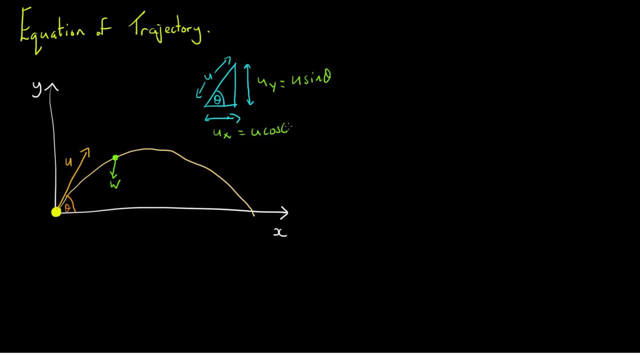 and u of x is equal to u cos theta And because of the weight acting only in the vertical direction, if we consider the horizontal sense, this will not change. So we can use speed equals distance divided by time to relate speed, distance and time. 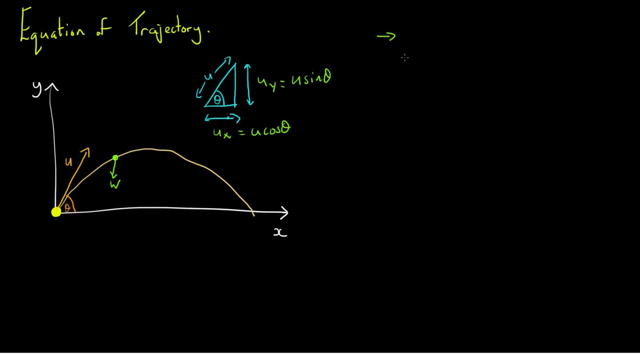 So for the horizontal speed, which is u cos theta, is equal to distance travelled, which is in a horizontal sense. so that means x divided by time. If I rearrange this for time, we end up with: t is equal to x divided by u cos theta. 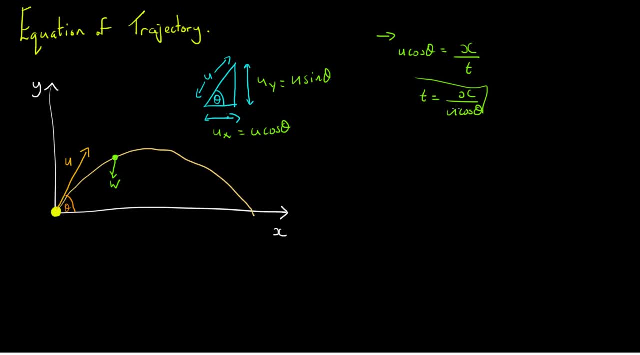 I'm going to use this extensively for the derivation. Okay, what about the vertical motion? Well, if I take that down here, a different colour. it's going to look like this: It's going to look like this: In this case, we do have a weight acting, we do have a force. 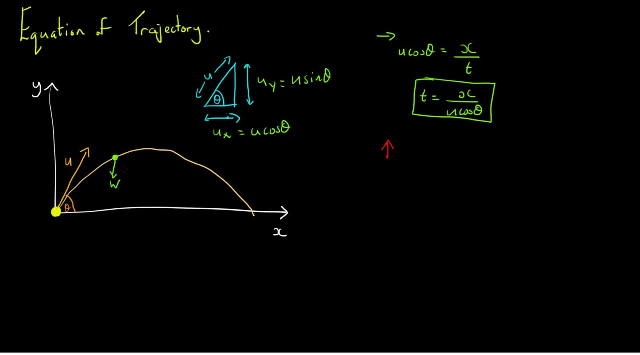 So, according to Newton's second law, we are going to experience an acceleration. And what is that acceleration? Well, the magnitude of the acceleration due to gravity close to the surface of the Earth is g, which has a value of 9.81 metres per second squared. 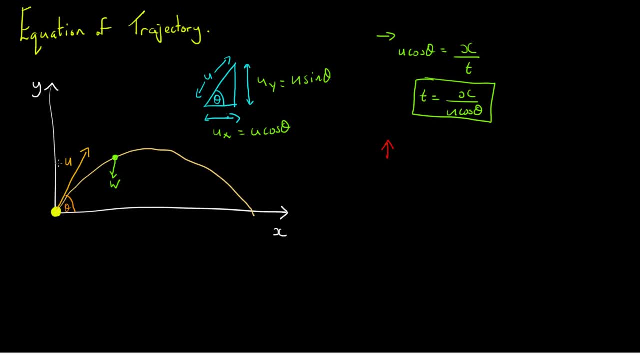 But because of the way we've defined our axes, we've said that y increasing is vertically upwards. So as acceleration points vertically downwards, acceleration is going to be minus g. Mark that with a line with two arrows. That's minus g. 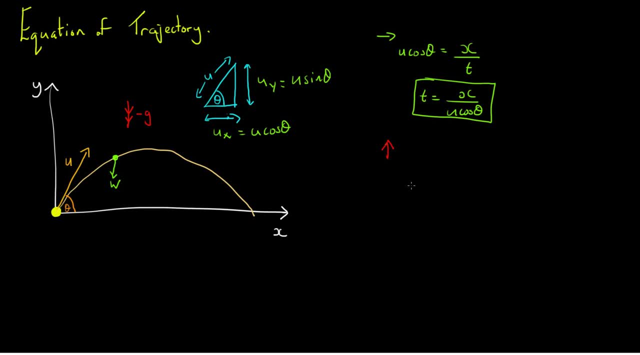 So, considering the vertical motion, we can use our Suvat equations to relate y, the height obtained, and time, And that's in the form of: s is equal to ut plus one half at squared, And we apply what we've currently got to this formula. 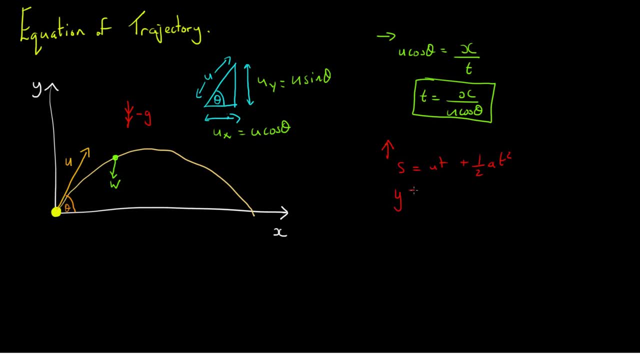 s is now no longer s, but it's y, the vertical height, And that's equal to u, which is the initial speed. but it's not the initial speed along this vector, it's in the vertical sense, which is u sine theta here. 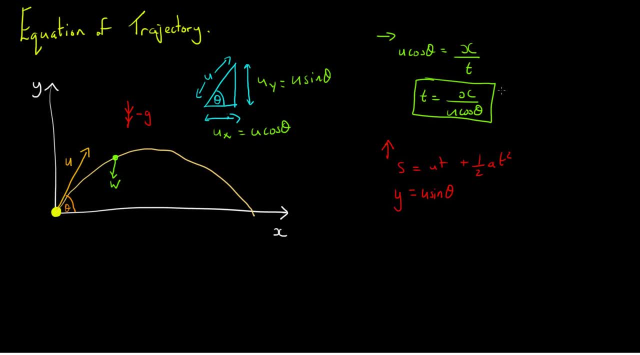 Now, instead of t, I'm going to replace that with this: what we rearranged from the horizontal motion. So we're going to times that by x divided by u, cos theta For the next term we've got. acceleration is not positive, it's minus g. 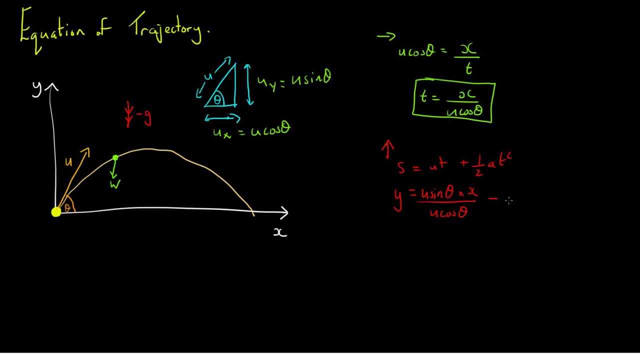 From our sine convention. So rather than plus, it's going to be minus. Acceleration is g And we've got t squared. Well, t squared is just this squared which, on the top, gives us x squared. We've got the two from the half. 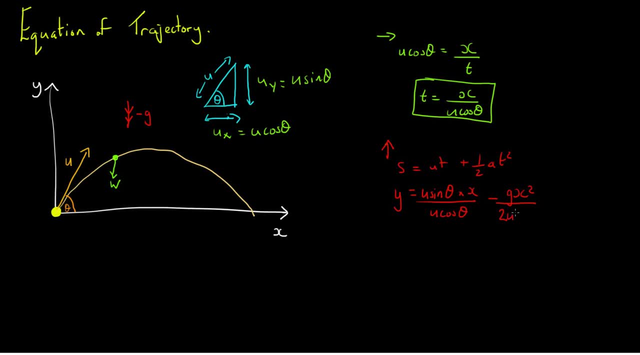 And then we've got u squared cos squared theta, just squaring that term there And if we tidy this up a bit, cancel the u's in the first term and recognize that sine theta divided by cos, theta is tan theta, we end up. 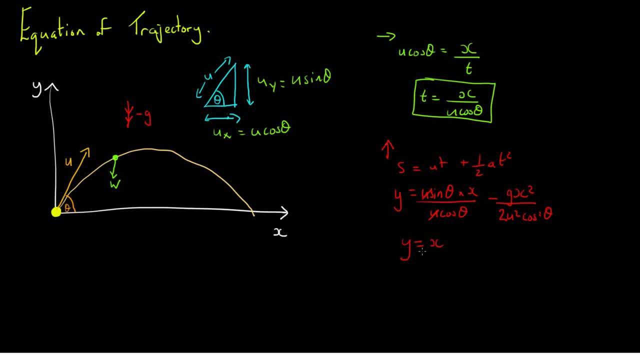 with our equation of trajectory, which is y is equal to x tan theta, minus g, x squared divided by two: u squared, cos squared theta. And this is our equation of trajectory. So, given a value of x, which is our distance from the origin in a horizontal sense, 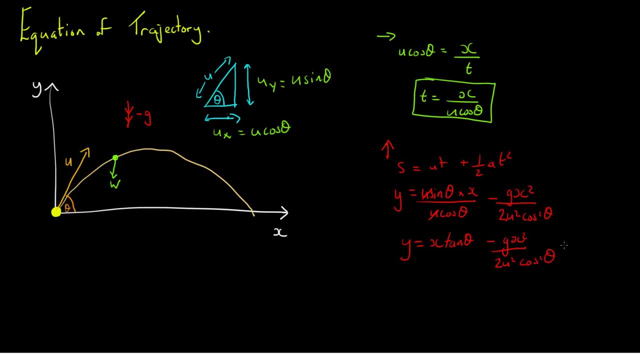 we're able to obtain our y value. Are we happy with this? Well, does it make sense that this is it an x term, an x squared term? even well, we have a parabola here. we have a curve, so we were expecting definitely a a squared term here. so we're we're reasonably happy with this, but we'll go on to. 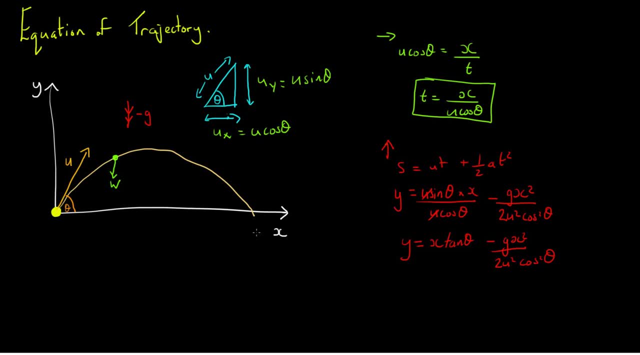 justify our expressions for for other things, and maybe i can convince you that this is definitely a sound formula. okay, so there's two things we generally want to do with with trajectories, first of which is to find the range, and that is defined as the distance from this point to this point, or the distance in the x direction. 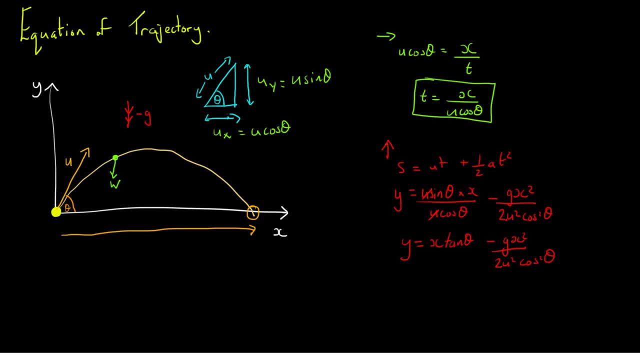 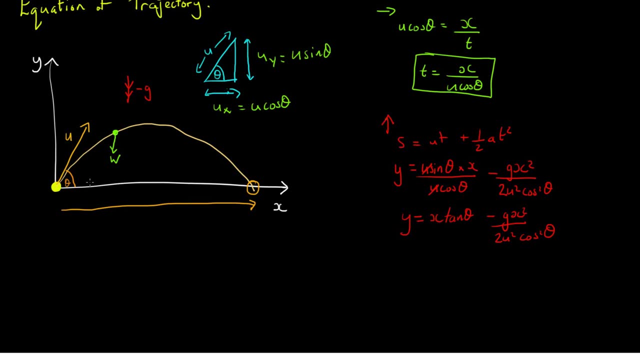 so let's do that first. um, how can we find that point using this formula? well, the first thing to recognize is due to our axes, the way we've defined them. this point will be at the point y equals zero. so if we substitute y equals zero into this formula and solve for x, we will obtain this. 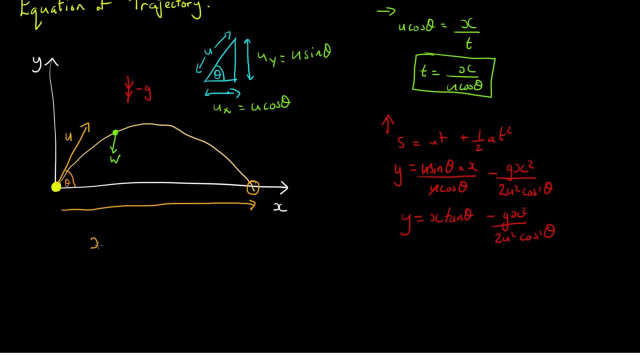 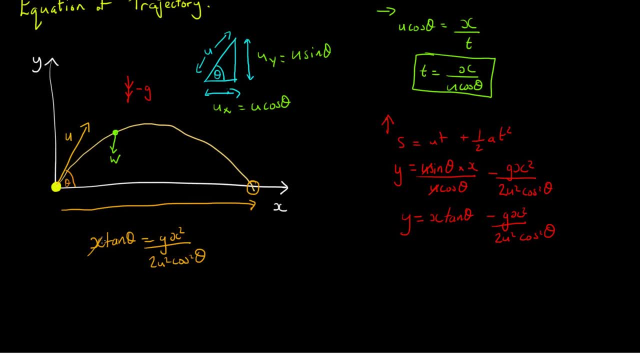 this term over to the other side. now i'm going to divide by zero. sorry, not divided by zero, divided by x, uh, and we're going to assume here that x is not equal to zero. we do not want this here. we don't want this trivial solution, because this will provide us uh, x equals zero, which is: 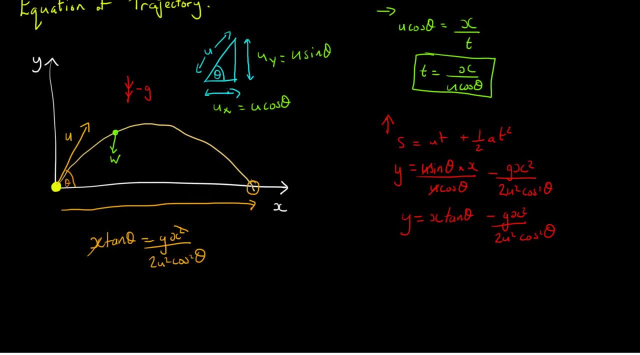 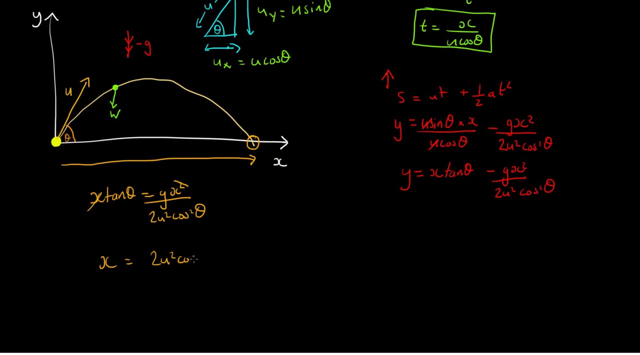 it's kind of pointless for our situation. we want to find this point here, so canceling that x, we're well justified. so if we rearrange this for x, we end up with x is equal to 2. u squared cos squared theta times, by tan theta, just taking this term up and then divided by g. now, cos squared times. 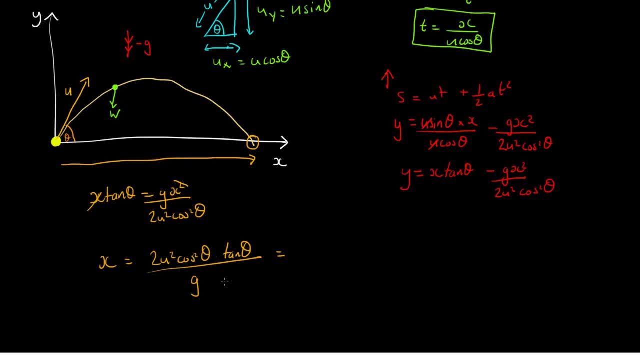 tan theta. well, tan theta is made up of sine theta divided by cos theta, so we've written that as that we'd have sine theta on the top and cos theta underneath, so i'm going to cancel that cos with this other cos, so we end up with 2? u squared: sine theta, cos theta. 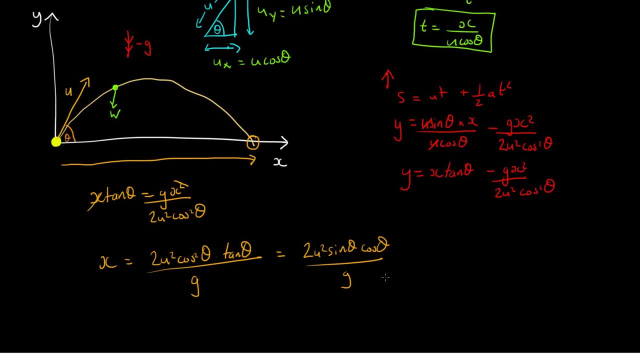 divided by g. and from your double angle formula, you should know that 2 sine theta cos theta is sine 2 theta. that can be written as: u squared sine 2 theta divided by g. okay, now are we happy with this? well, does it make sense that if we increase our speed, that we launch? 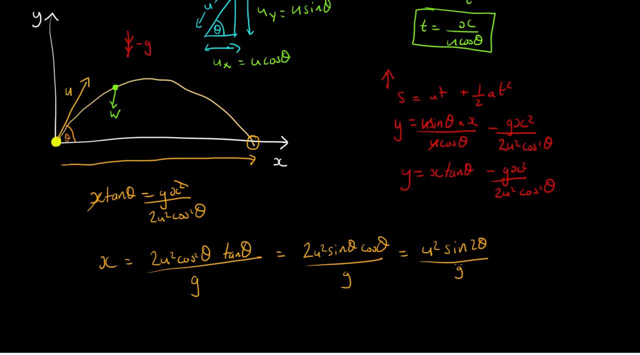 out we go further. well, yes, it does. does it make sense that if we increase the gravitational field strength, that we don't go as far? well again, yes, um, to justify this: sine 2 theta. why is it sine 2 theta? well, the maximum value for sine of some angle is: is that sine of 90? for our first solution? 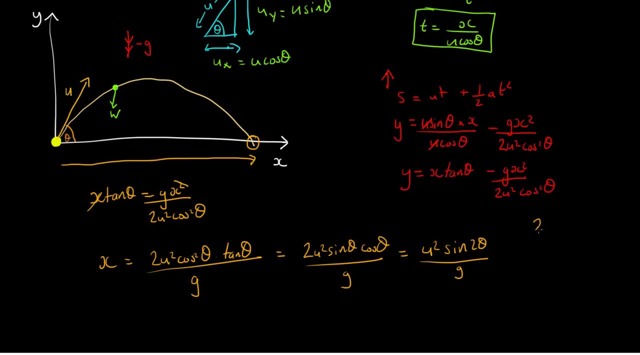 so what we're saying is to get a maximum for this. we say that 2 theta is equal to 90 degrees, because sine varies from plus 1 to minus 1, and we want to get plus 1 for our maximum. so we can say that theta for our maximum value is 45. 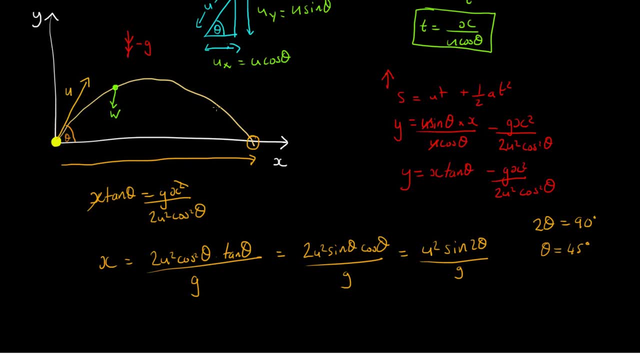 degrees again. does that make sense that the furthest we travel, the furthest distance if our angle is 45 degrees? well, yes, it does. if we pointed this vector vertically upwards, particle would go up, turn around and come back down again. and we pointed it horizontally, if it wasn't allowed to roll, this ball wouldn't travel anywhere. so our maximum range is obtained. 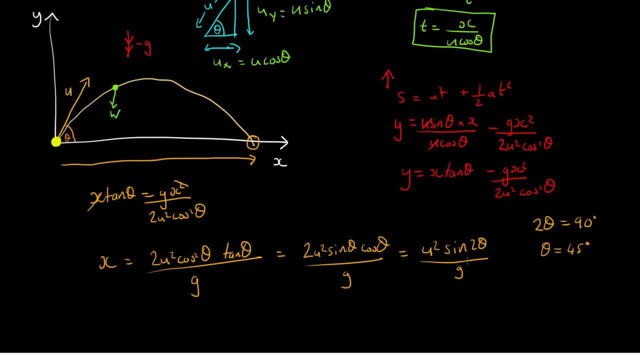 at an angle of 45 degrees, halfway between. so we're happy with this. but what about finding this height, the maximum height obtained? it's the other thing that we normally want to do. well, there's first of all- I want to find this, this distance here, this X distance. there's two ways we can do that. we can: 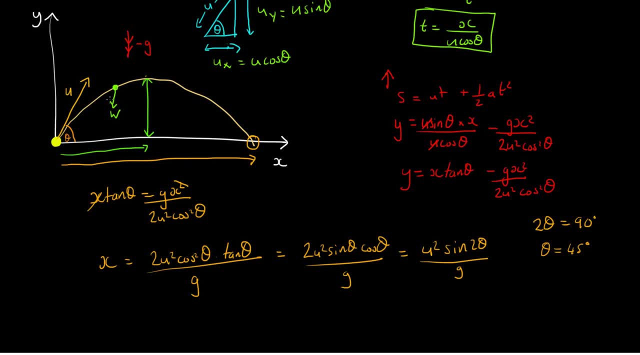 take if we can see that this is symmetrical, about this line- which is our maximum point because it is a parabola- and say that the distance from here to them halfway point is exactly halfway between here and the end point. so we can just divide this distance by 2. or, if you don't trust me, if you: 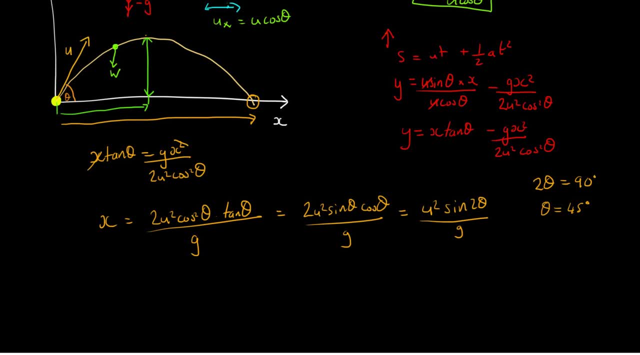 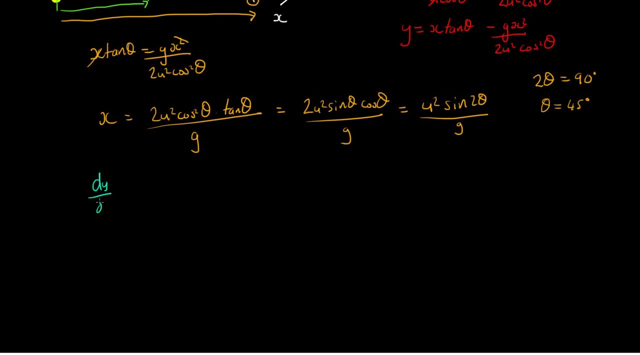 take the derivative of this expression and I'll do that down here. we take dy, dx of this expression end up with dy. by dx is equal to. if we differentiate X, tan theta with respect to X, not with respect to theta, we just end up with tan theta. tan theta is just a number. however, if we differentiate the 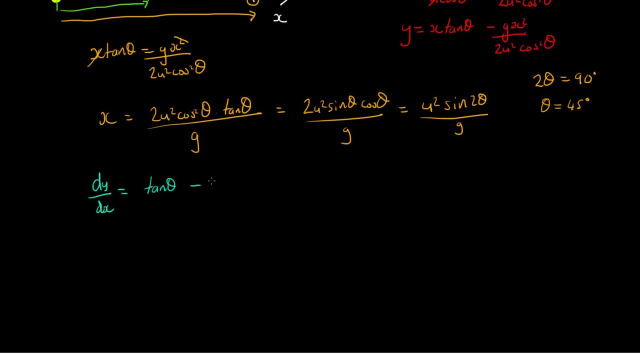 second term. we end up with minus G. X divided by u squared cos squared theta, the two. when we differentiate X squared, we get 2x. the two is cancelled with the two underneath. so we end up with this term. now, what can we do with dy dx to find this point? well, at dy dx, well do dy dx. 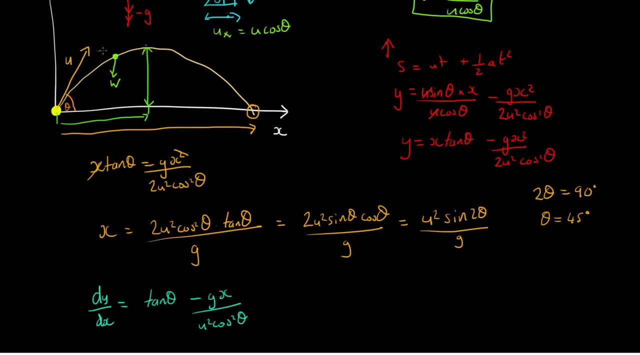 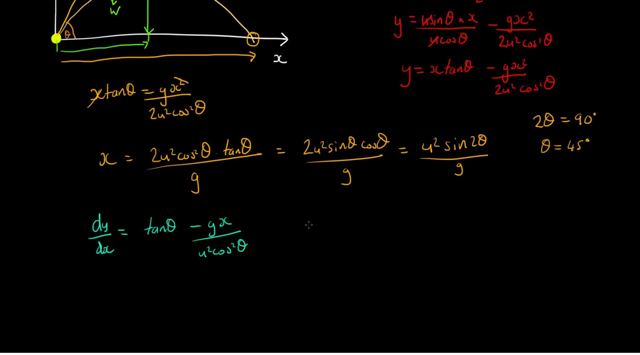 represents the, the gradient of this curve, and at this point we draw a tangent to the line. you can see that the gradient of that is 0. so dy by dx at that point is 0, and so what we can do is we can set this expression equal to 0. so we end up with G X divided by u squared cos squared theta. 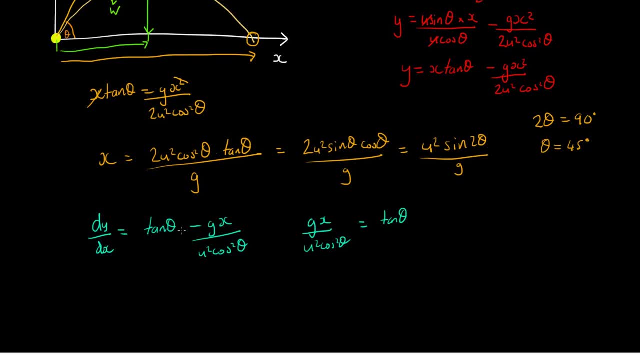 is equal to tan theta. second this to 0, moving the other term over. we multiply u squared cos squared theta up and divide by G. we end up with X is equal to tan theta times by u squared cos squared theta divided by G. now, this is exactly the same as this expression, apart from we've 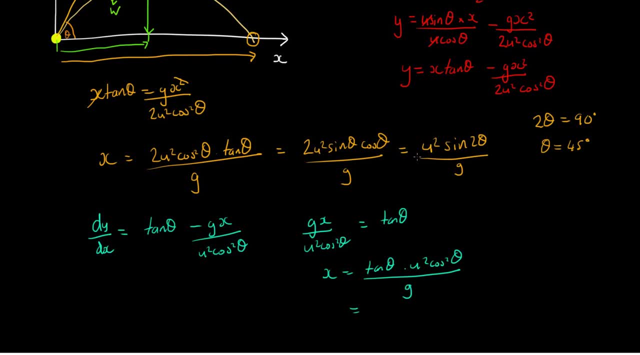 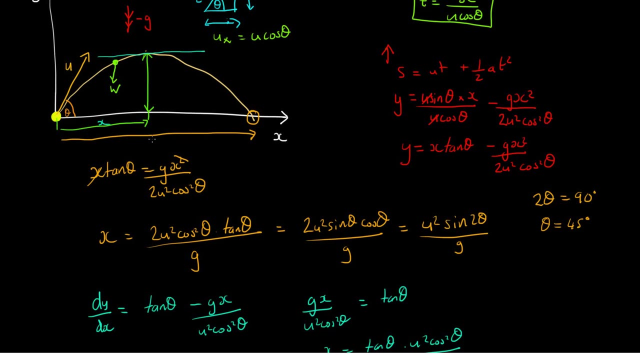 got half as much of it. so this is equal to half of our result that we had over here, and so you should have trusted me. we end up with u squared sine 2 theta divided by 2 G. so, yes, we have justified that this X distance here is equal to half of the X distance from here to here. the 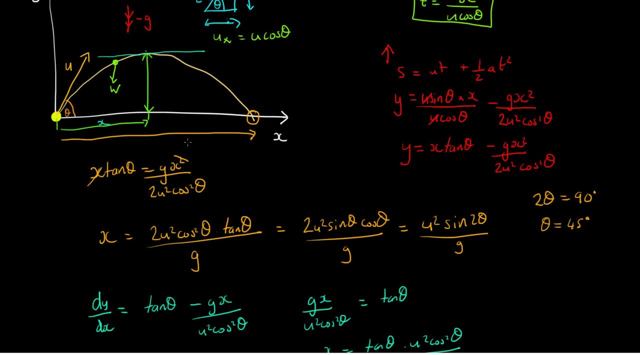 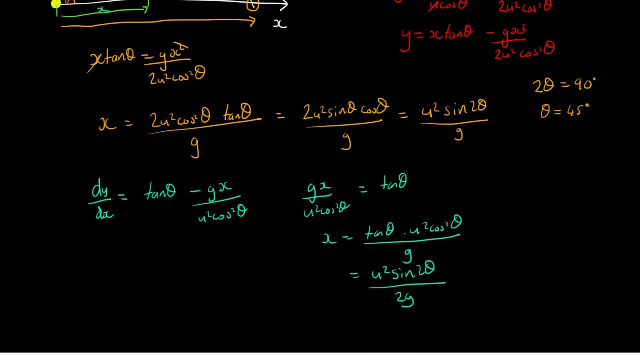 range of the expression. but what about the calculating this height? well, now we have a value of X. it's just a matter of substituting this value of X into our expression to get a value of Y. so if we do that, we end up with Y is equal to half of the X distance from here to here. 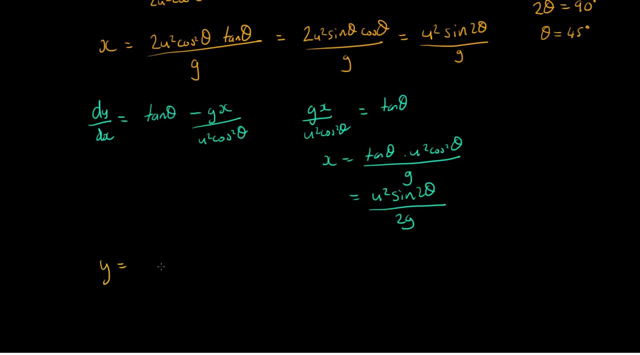 so if we do that, we end up with: Y is equal to X tan theta. X is now this: so it's equal to u squared sine, and instead of- actually instead of sine- 2 theta, I'm going to write this as 2 sine theta, cos theta it's equivalent, and it just makes it a little bit easier for doing the manipulation. 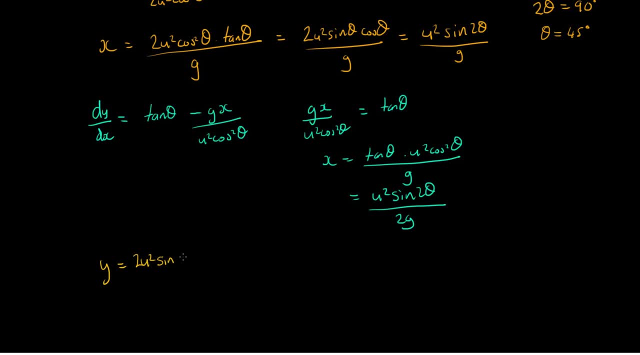 so this ends up being 2 u squared sine theta cos theta divided by 2G. again, we're going to cancel the twos here and here times by tan theta. This was our x value, if you remember. Now, if we look at our next term, we end up with minus g over 2u squared cos squared theta times by x squared. 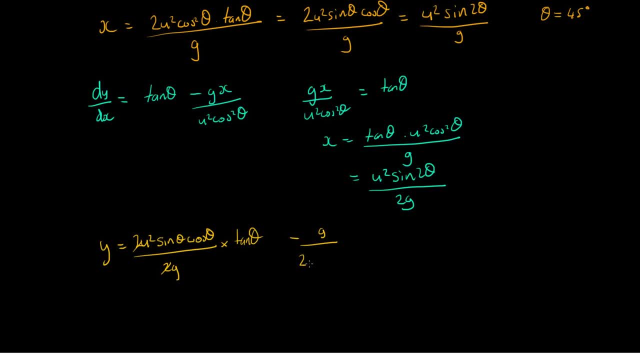 So minus g divided by 2u squared cos squared. theta times by x squared. Well, if this is x, then x squared is just a matter of taking the product of this, which is going to be u, to the fourth power Times by sine squared theta cos squared. theta divided by 4g squared. 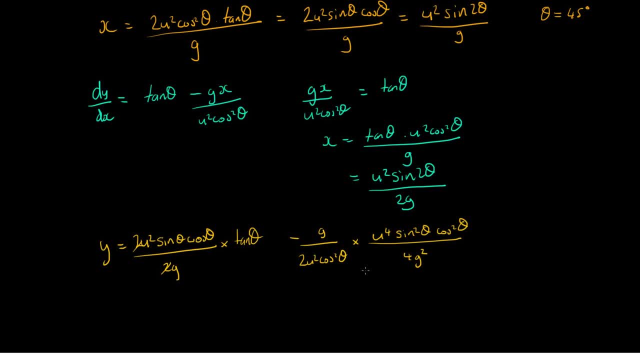 doubling squaring this term underneath. If we actually sine 2 theta is 2 sine theta cos theta. so we're going to have an extra 4 coming out the front if we square that 2.. Sorry for that. This 4 will cancel with this 4.. 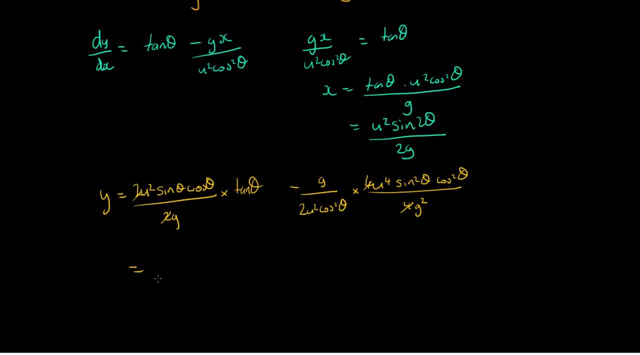 And then if we just write this out again neatly now we end up with on the left-hand side, we have u squared sine theta, cos theta, tan theta divided by g. And if we deal with this on the right-hand side, well, we have cos squared theta here. 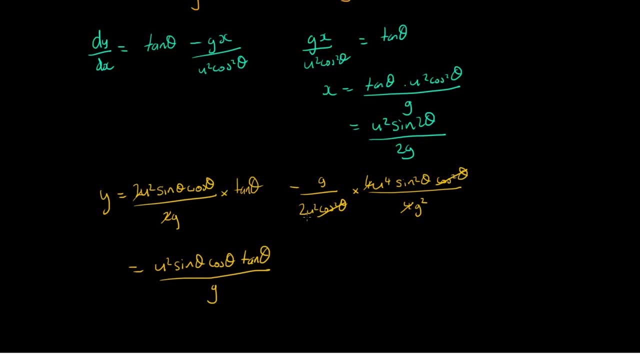 and that's going to cancel with that cos squared theta here. We have u squared theta here, so that's going to cancel with the u to the fourth power to give u to the second power. So this ends up being minus g, u squared. 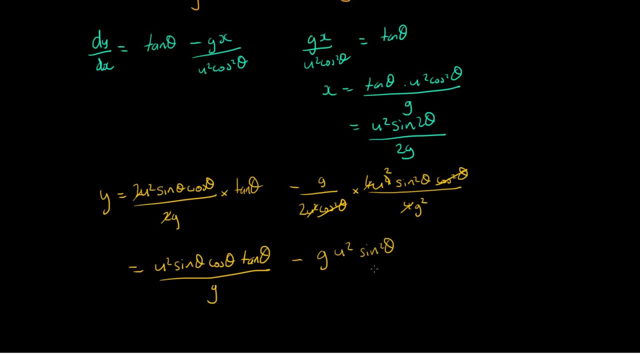 So we're going to have u squared, sine squared theta divided by g squared, There's 2, and there's 2 over here. This squared cancels with this g Sine theta, cos theta, tan theta. Well, tan theta is sine theta divided by cos theta. 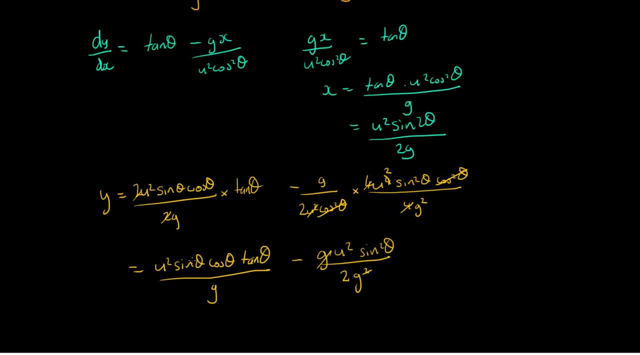 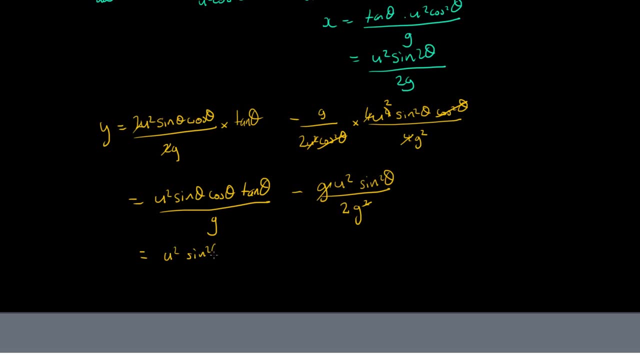 so that cos theta is going to cancel with this cos theta, and the sine is going to end up being a product with this sine. So we're going to end up with u squared sine squared theta divided by g minus u squared sine squared theta divided by 2g.